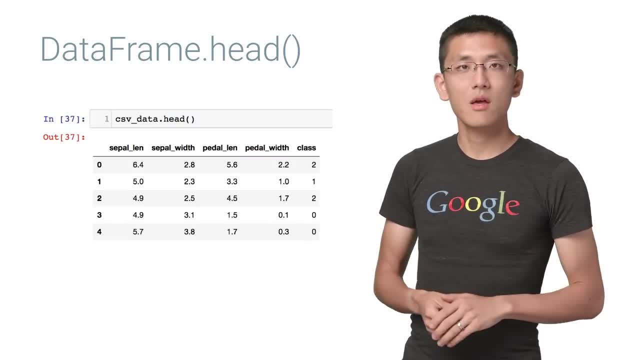 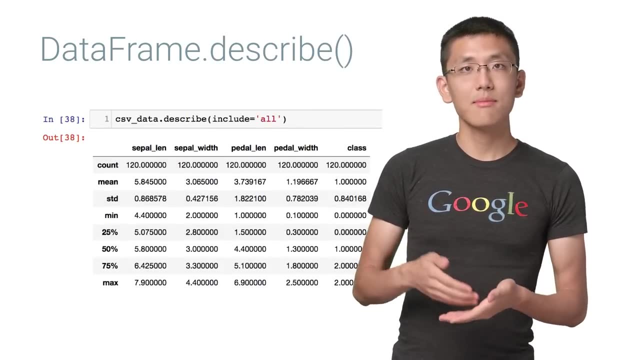 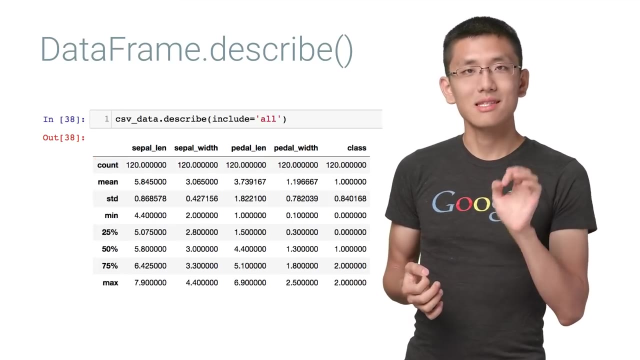 This can be thought of as essentially a table or spreadsheet. We can take a quick glimpse of our data by calling head on our data frame. Data frames have rows of data with named columns, which in pandas, are called series. For me, one of the nicest things about data frames is the describe function. 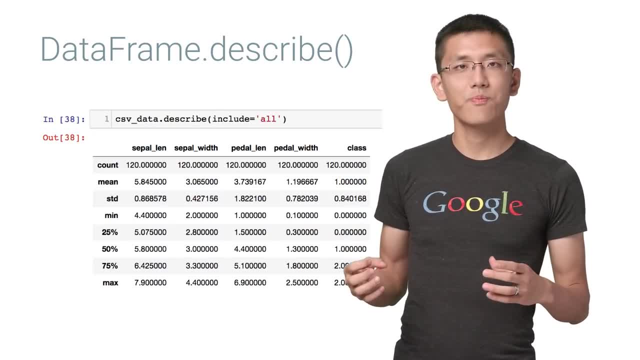 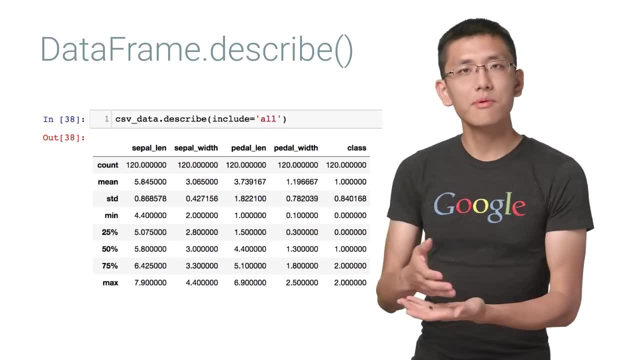 which displays a table of statistics about your data frame. This is super useful for sanity checking your dataset, seeing if the distribution of your data looks reasonable and whether the properties are what you expect them to be. I also sometimes will use pandas to shuffle my data. 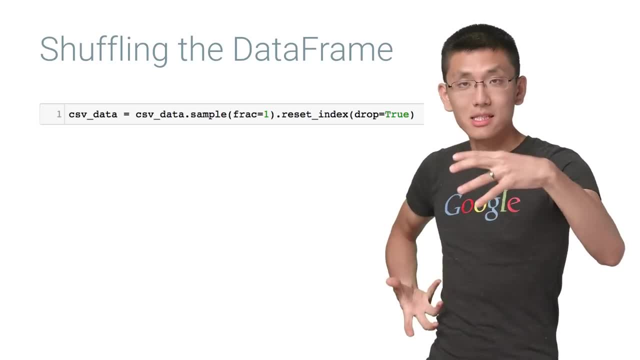 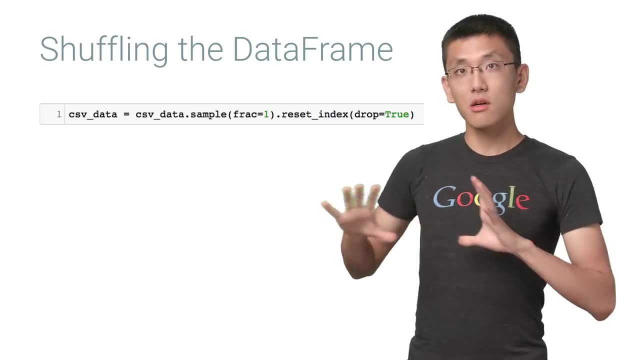 This can be useful in situations where you want to shuffle the entire dataset rather than merely having a lookahead buffer as you extract data out. For example, if your data is not shuffled at all and is in fact already sorted, you'd want to give it an extra good mixing. 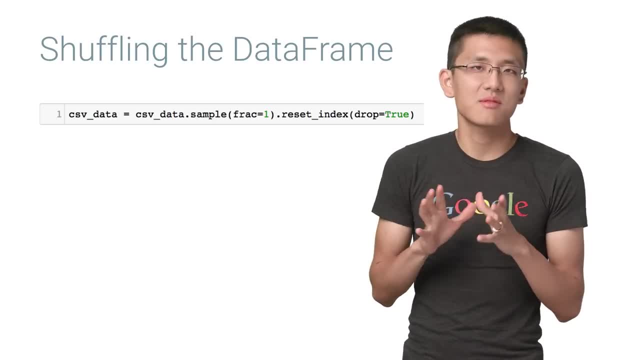 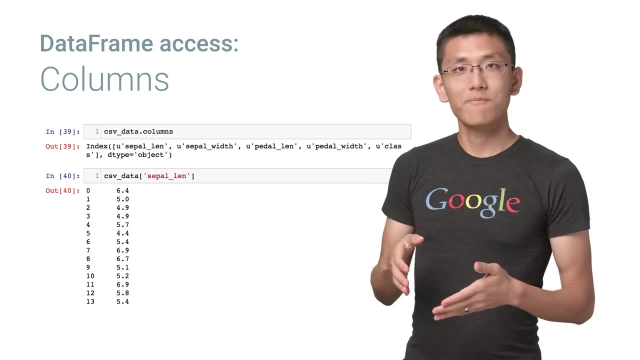 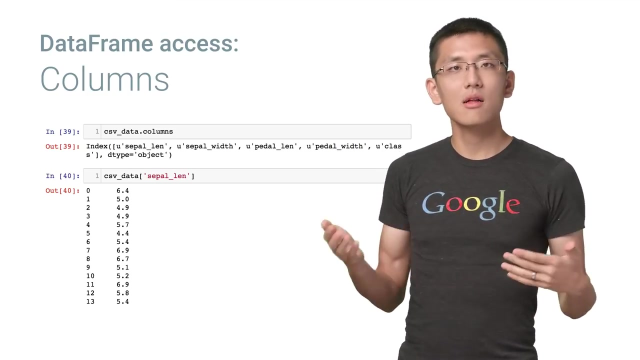 However, for truly huge datasets, it's possible that this may be impractical without more sophisticated approaches. To access a particular column of a dataset, use bracket notation to pull out that column, passing in the name of that column. If you're wondering what the possible column names are, you can look back at the output of. 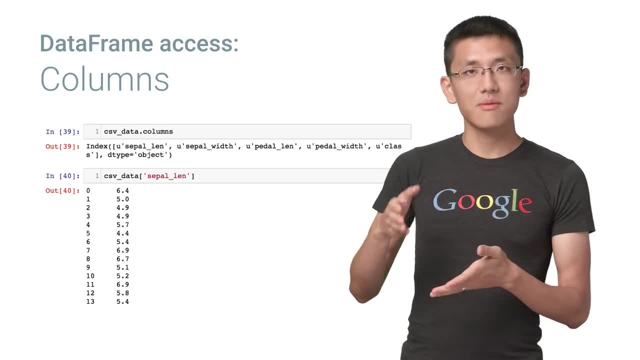 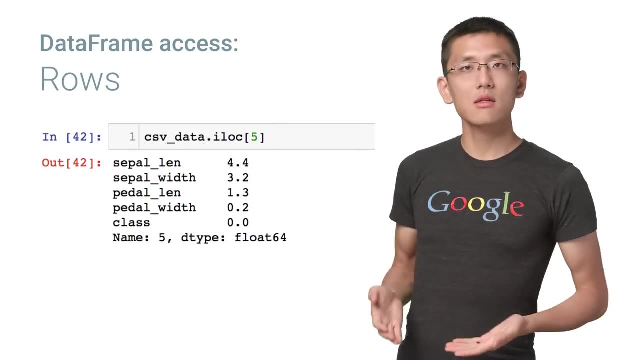 describe or use df or dataframecolumns to access all the columns in the data frame as an array. If you can access data column by column, then the next thing you'll want to know is how to access it by row. Accessing rows of data frames is 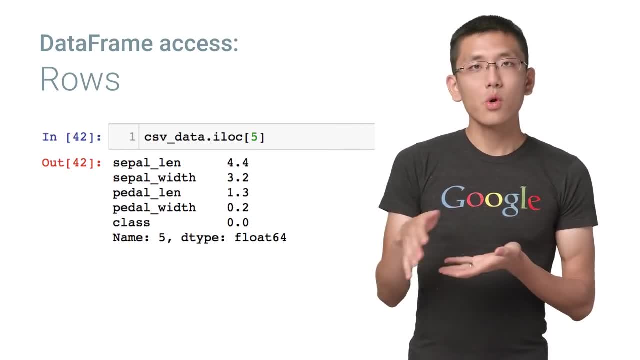 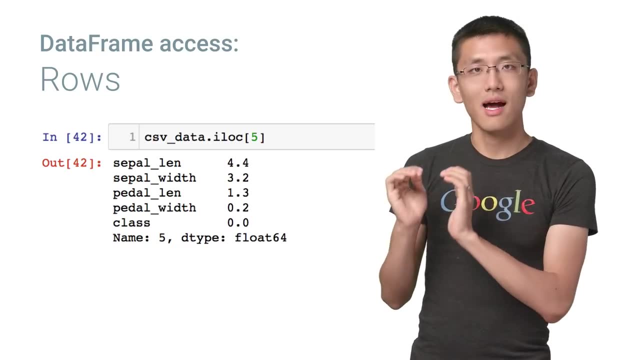 a little bit different than from columns. For example, if we want the row with an index i of a given data frame, we can use iloc or i location. index location at: i. Keep in mind that pandas operates on a zero-based indexing system. 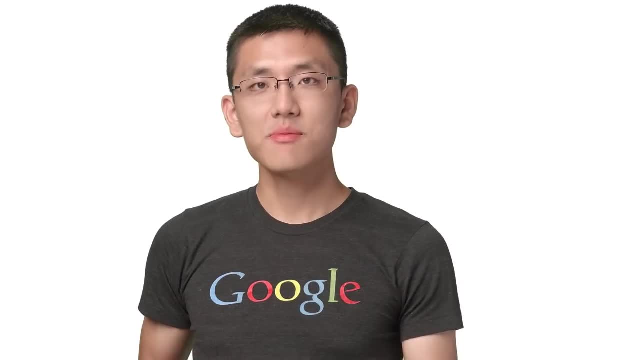 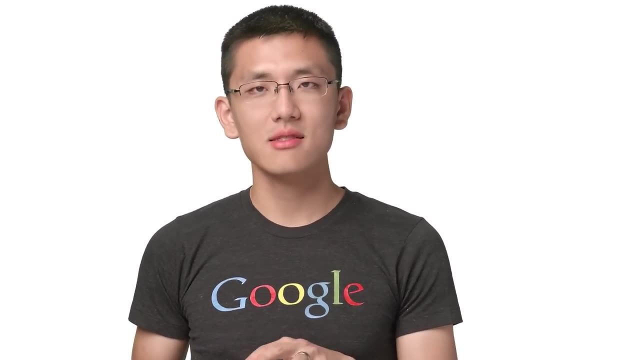 so the first row is actually indexed zero. Sometimes you may want a particular row and column. Because rows and columns are accessed differently, we'll need different techniques to get that done. In particular, if you want row 5 of a column called name, 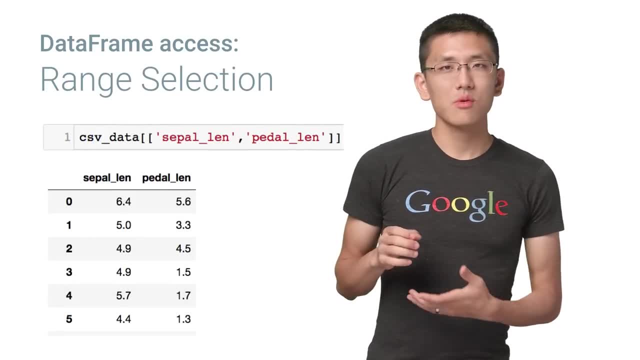 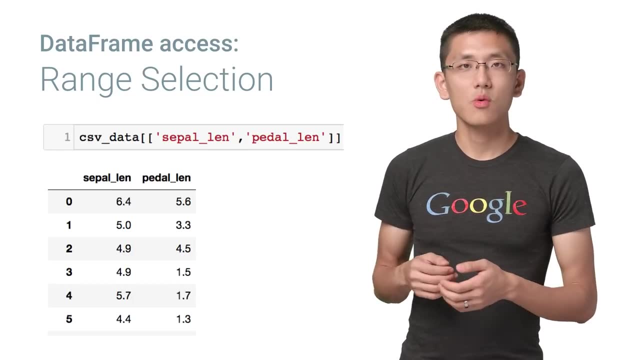 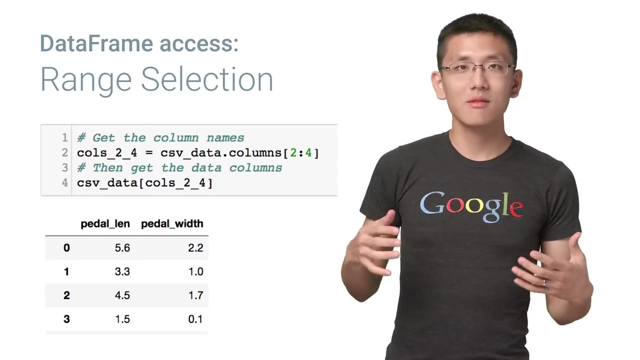 you would use something like this. And where things get much more interesting is when you want to get a whole range of columns and rows On the column side. the way to get multiple columns is to pass in an array of those column names If there are many, many columns and you don't want to type them all out.